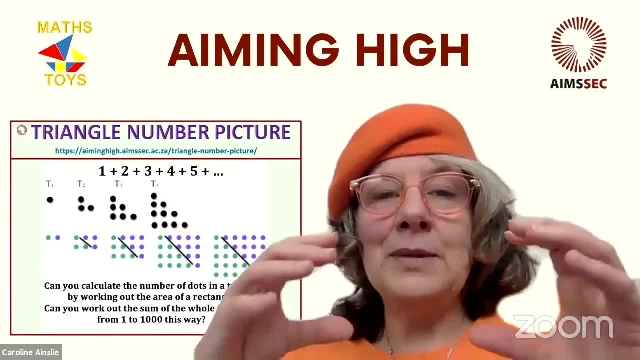 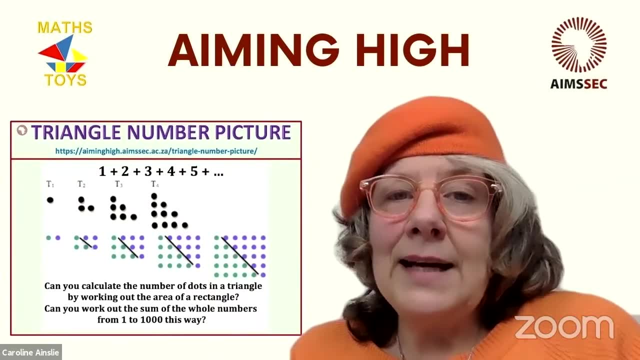 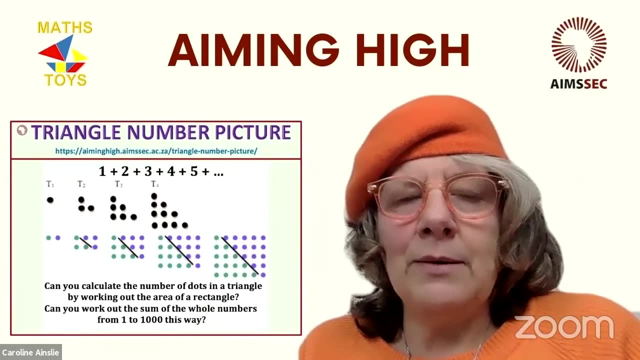 If you put two of them together, one upside down and attached to each other so that they follow the same rows, you get a rectangle. Now, this isn't the cut a triangle in half thing that I did when I was in school: One triangle's there and the other triangle's there. 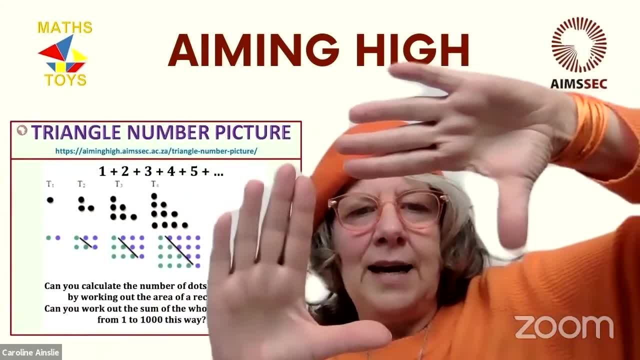 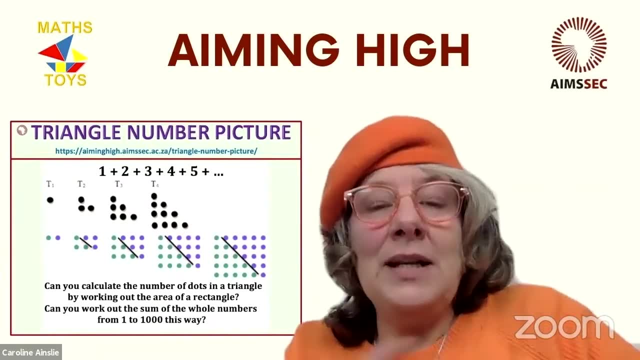 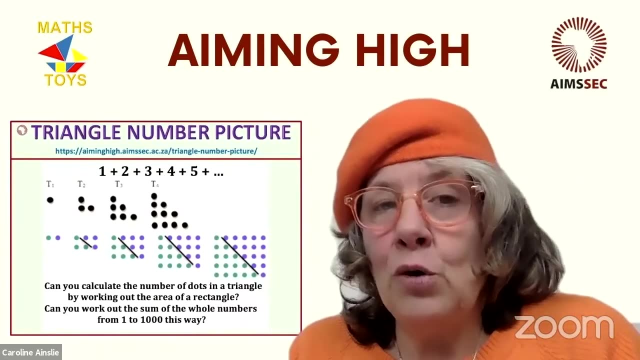 so they're not joining like that, they're joining slightly offset. Now it's fascinating and the thing is, you can just get into doing this activity by purely drawing. You don't have to do any algebra, You don't have to write anything down on paper apart from record what you're doing. 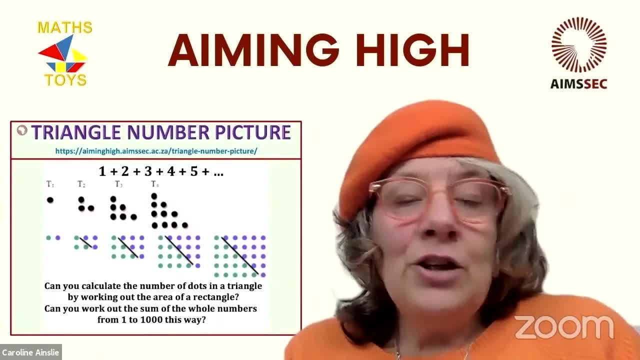 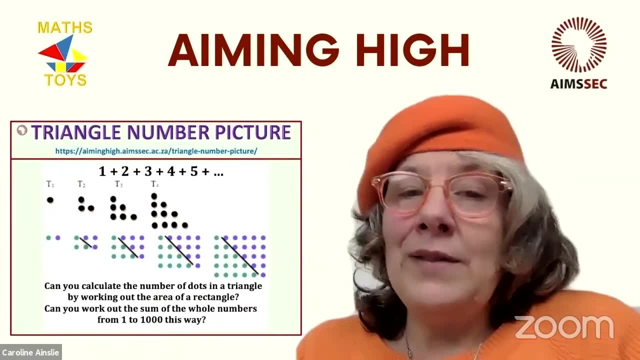 in whatever way you want to record it, you can do it that way. I had the questions. Can you calculate the number of dots in a triangle by working out the area? The area, in case you've forgotten, is the length times the height. So how would you use that? 2 by 3, 1 by 2?? Do you want to do that spell by yourself to put extra impres prisoner? How would you do that? How would your practical method be? Okay, in the comments you've got the answer, but how would you use that? 2 by 3, 1 by 2? How would you use it? 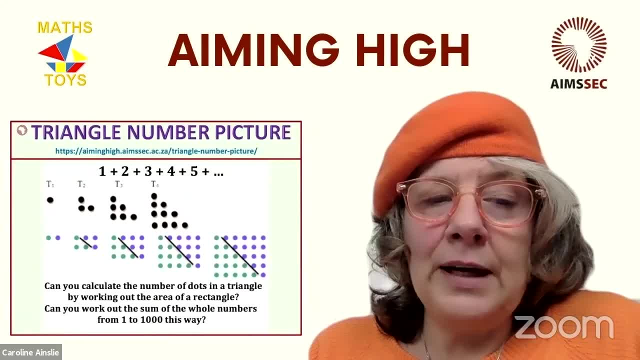 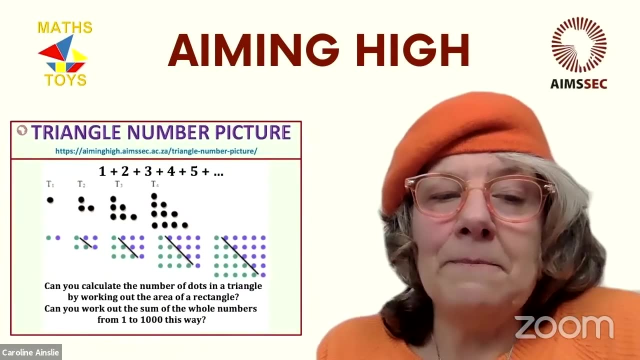 So how would you use that? two by three, one by two? How would you do that? So that's first pause for thought, And then can you work out the sum of the whole numbers from one to one thousand in this way? So that would be T. I guess it would be T one thousand. 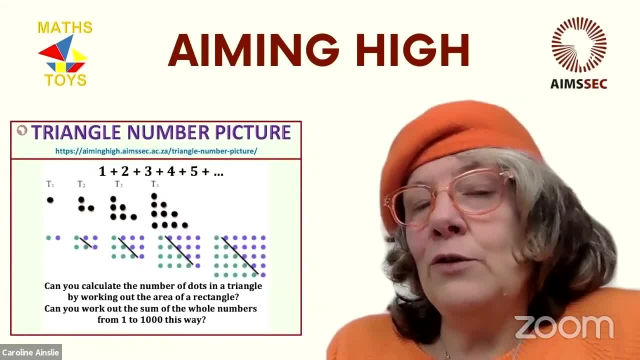 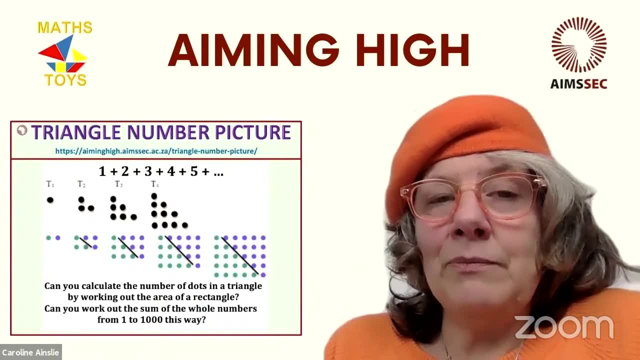 So just have a play with it. Have a play with, first of all, do it with images and dots And then go on to doing it. see if you've got some people with more experience in your household. go on to do it algebraically. 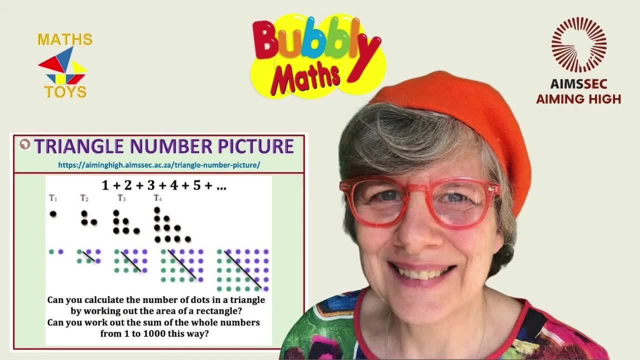 There is a link to the home learning and the teacher guide, plus more activities in the description. Please also support AIMSEC through the GoFundMe link given Subscribe, comment and ding the notification bell to make sure you don't miss our latest videos.